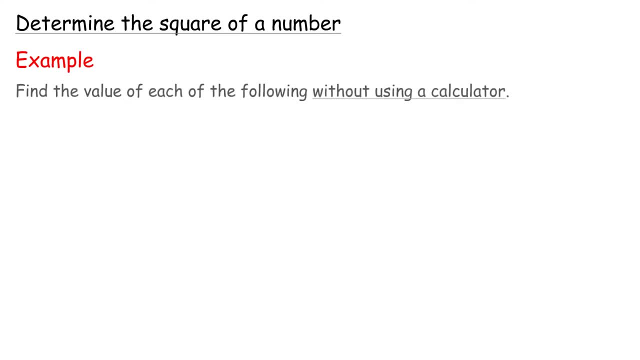 Determine the square of a number. Example: find the value of each of the following without using a calculator: 6.. Solution: a: 6 squared equals 6 times 6. equals 36.. b: 3 over 4 squared equals 3 over 4 times 3 over 4 equals 9 over 16.. 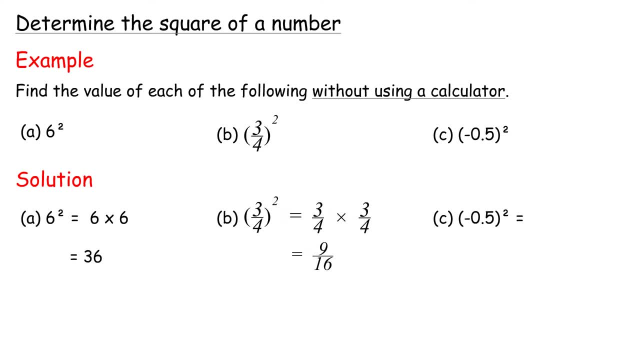 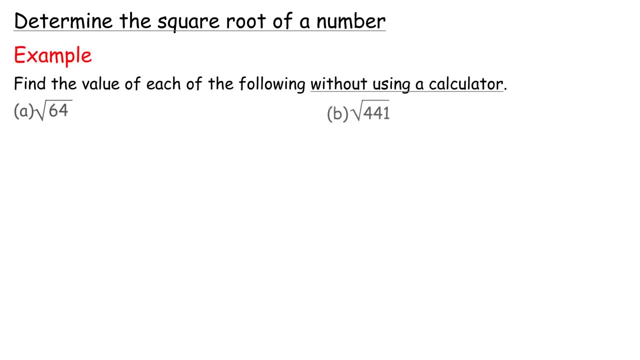 c: Negative 0.5 squared equals negative 0.5 times negative 0.5 equals 0.25.. Determine the square root of a number. Example: find the value of each of the following without using a calculator: 6.. Solution: a Square root of 64 equals square root of 8 times 8 equals 8.. 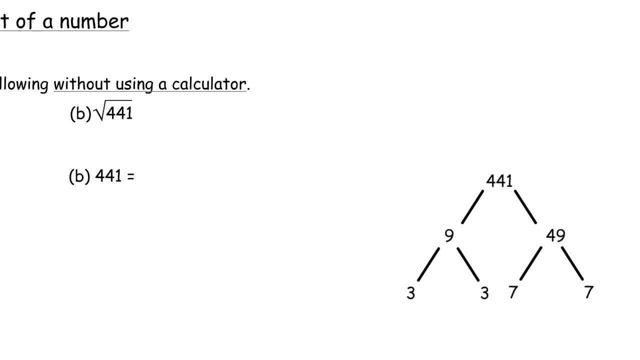 b 441 equals 3 times 3 times 7 times 7. equals 3 times 7 times 3 times 7 equals 21 times 21.. c: Negative 0.5 squared equals also negative 0.5, because there is a final value of 5 times 3 times 8.. 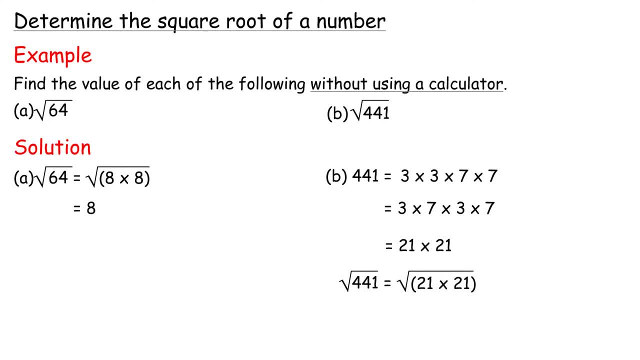 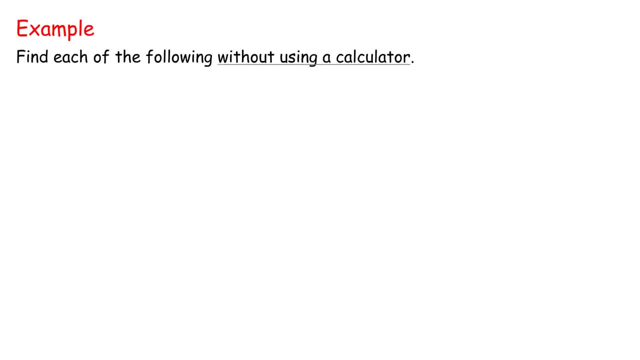 21, equals square root 21 times 21, equals 21.. Example: find the value of each of the following without using a calculator Solution: a square root of 4 over 25, equals square root of 2 over 5, times 2 over 5,. 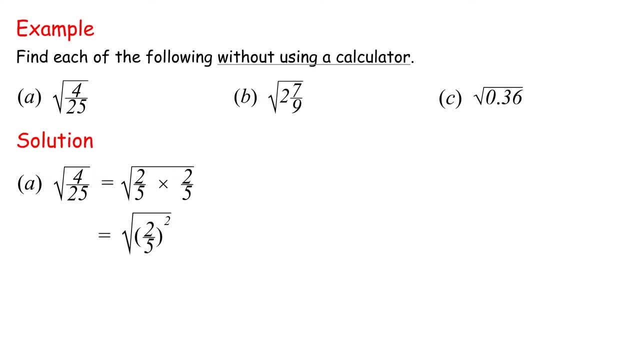 equals square root of 2 over 5, square equals 2 over 5.. b, square root of 2 and 7 over 9, equals square root of 25 over 9,. equals square root of 5 over 3, times 5 over 3, equals square root of 5 over 3, square equals 5 over 3.. 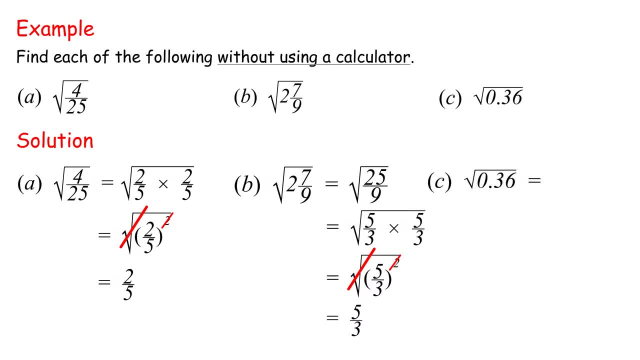 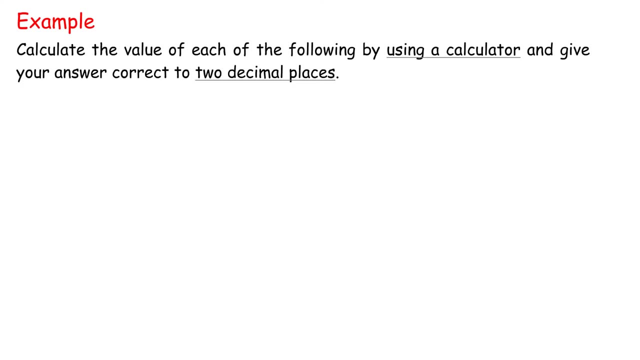 c. square root of 0.36,. 6 equals square root of 0.6 times 0.6 equals square root of 0.6. square equals 0.6. example. calculate the value of each of the following by using a calculator: 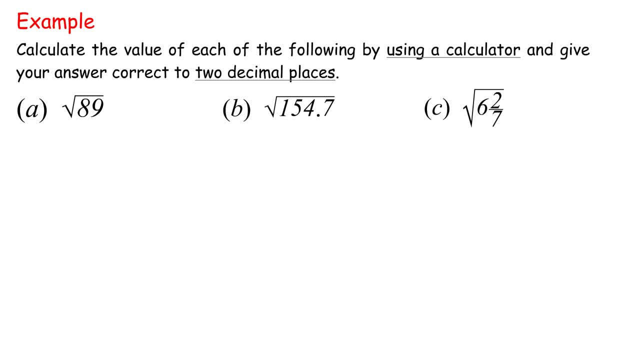 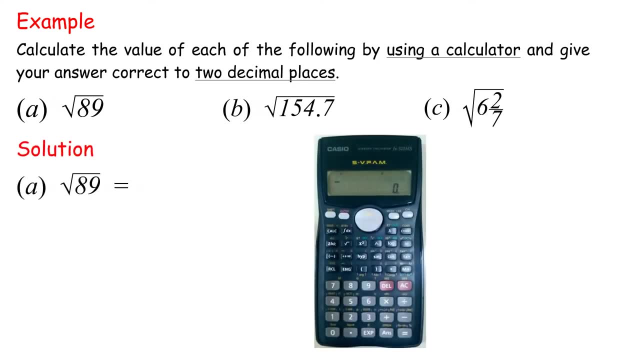 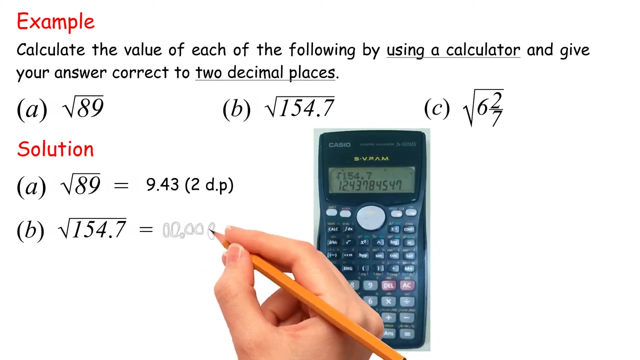 and give your answer correct to two decimal places. solution: a: square root 89: 0.6 equals 9.43 in two decimal places. b- square root 154.7 equals 12.44 in two decimal places. c- square root of 6 and 2 over 7. 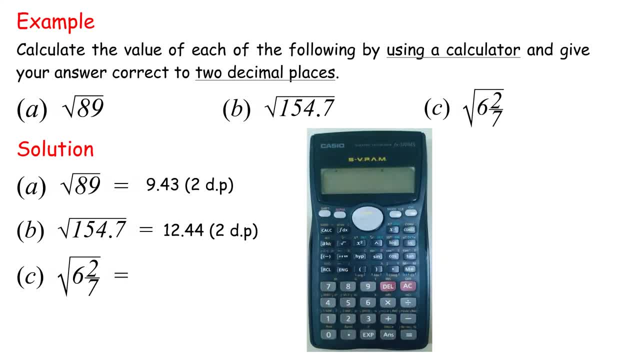 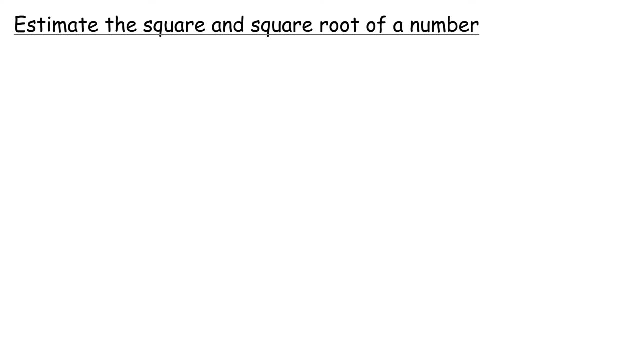 0.6 equals 2.51 in two decimal places. estimate the square and square root of a number. if we do not have a calculator and want to roughly know the value, we estimate. example: estimate the value of a, 27.5 squared b, square root of 54.. 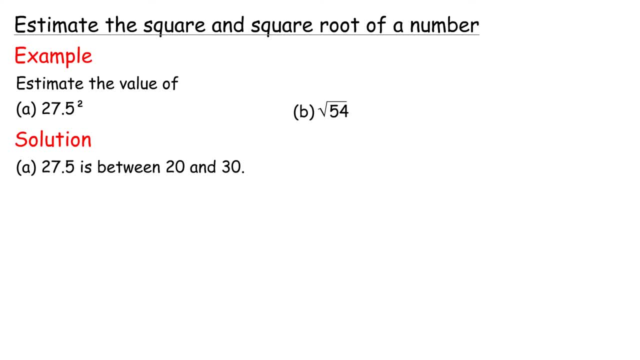 0.6 equals 3.00 in two decimal places, b square root of 1.5. 0.6 equals 3.00 in two decimal places, b square root of 6.. 0.6 equals 3.0 in two decimal places. a solution a: 27.5 is between 20 and 30.. 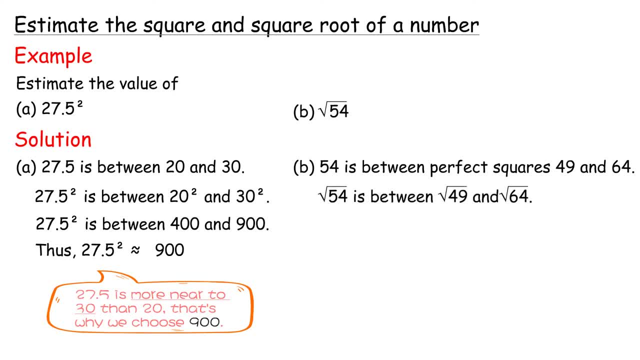 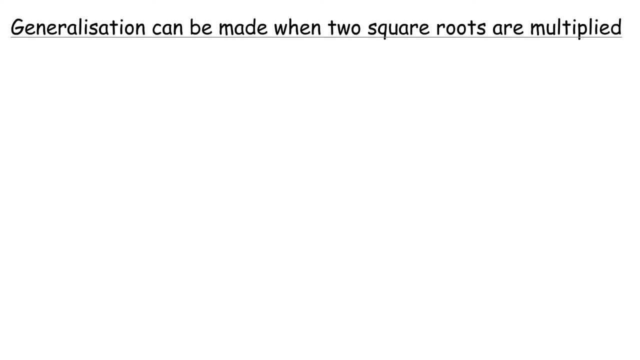 root of 54 is between square root of 49 and square root of 64. That is, square root of 54 is between 7 and 8.. Thus, square root of 54 approximate to 7.. Generalization can be made. 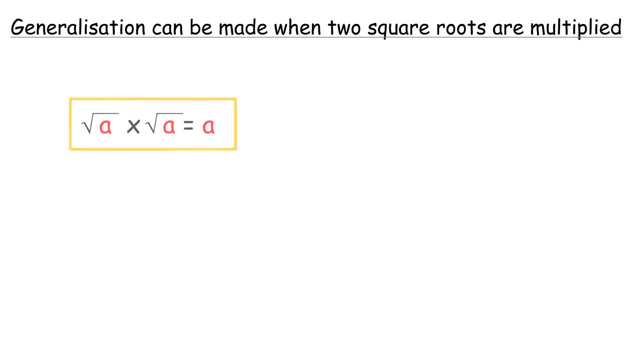 when two square roots are multiplied, The product of two equal square root numbers is the number itself, that is, square root of a times square root of a equals a. For instance, square root of 2 times square root of 2 equals 2.. The product of two different square root numbers is the square 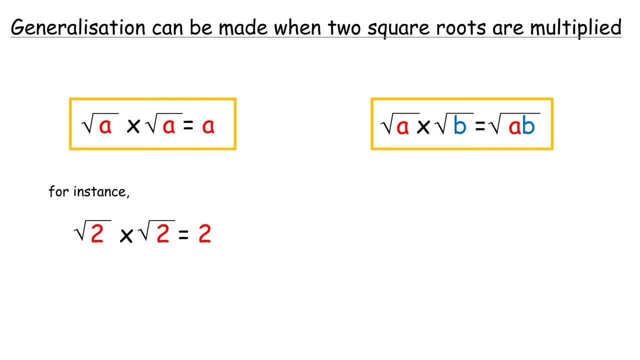 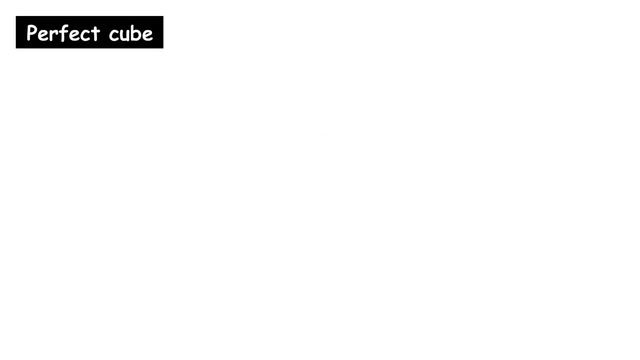 root of the product of the two numbers, that is, square root of a times square root of b. equals square root of a. b, For instance, square root of 2 times square root of 3.. equals square root of 2 times 3. equals square root of 6: 3.2. cubes and cube roots: perfect cube. 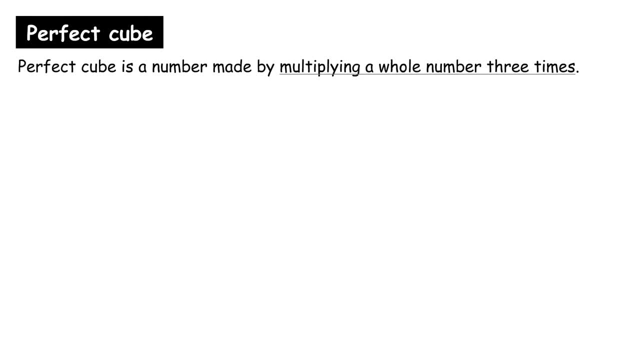 perfect cube is a number made by multiplying a whole number three times. for example, two cube is two repeated multiply for three times. three cubed is three repeated. multiply for three times determine whether a number is a perfect cube. we can also use the method of prime factorization. 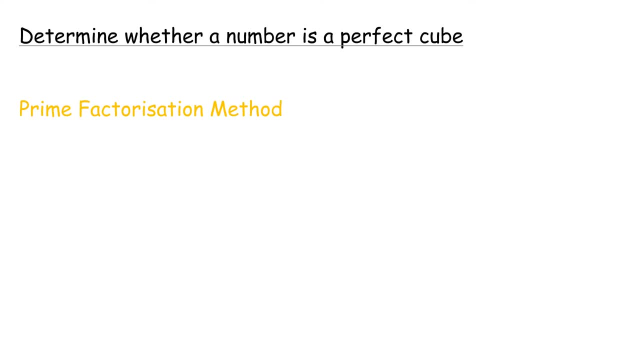 to determine whether a number is a perfect cube in this method, if the prime factors can be grouped into three identical groups, then the number is a perfect cube. example: determine whether each of the following numbers is a perfect cube: a 64 b 240. a 64 b 240. 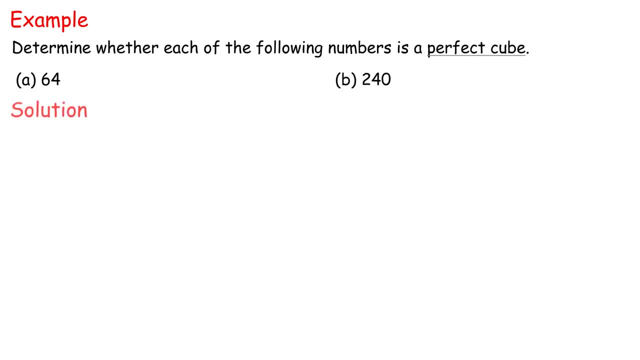 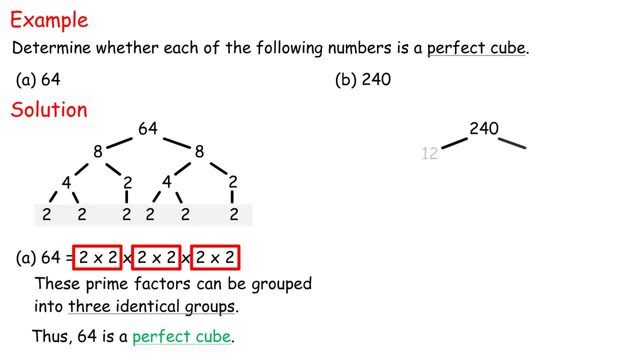 these prime factors can be grouped into three identical groups. thus, 64 is not a perfect cube. b 240 can be divided by 12 and 20, 12 can be divided by four and three, and 20 can be divided by four and 5. 4 can be further divided by 2 and 2, 240 equals 2 times 2 times 3 times 2 times 2 times 5. since these 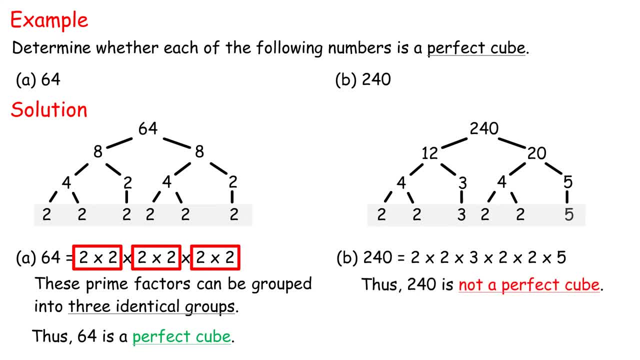 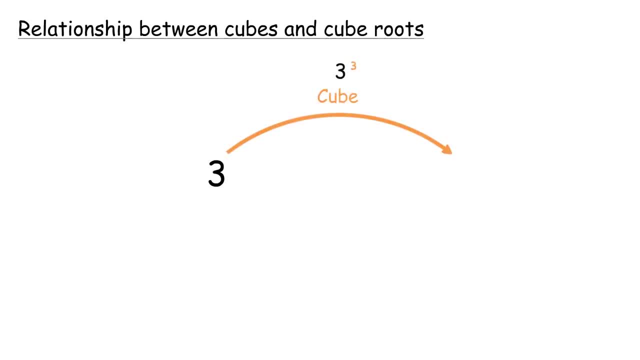 prime factors cannot be grouped into three identical groups. thus 240 is not a perfect cube. 3 cubed equals 3 times 3, times 3, equals 27.. Cube root of 27 equals 3.. Determine the cube of a number. 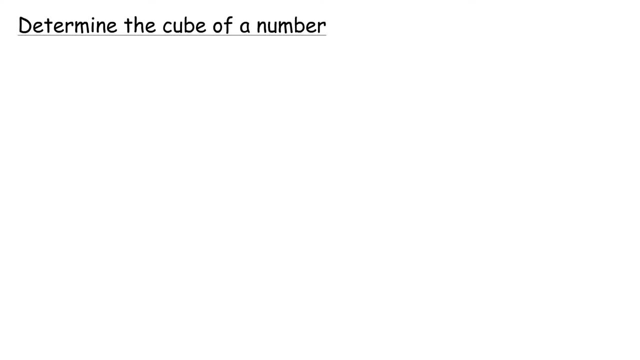 Example: Find the value of each of the following without using a calculator: 4 cubed equals 4 times 4, times 4, equals 64.. cube equals 0.2 times 0.2, times 0.2, equals 0.008.. 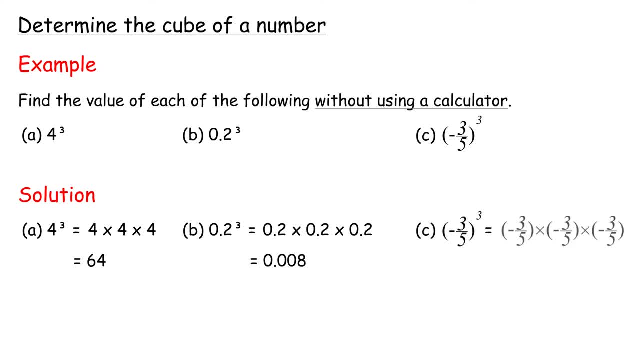 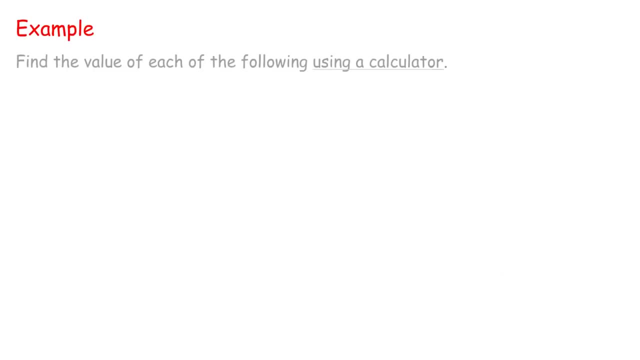 C. Negative 3 fifths cubed equals negative 3 fifths times 3 fifths negative. three-fifths times negative three-fifths equals negative twenty-seven. one hundred twenty-five Example: Find the value of each of the following using a calculator. 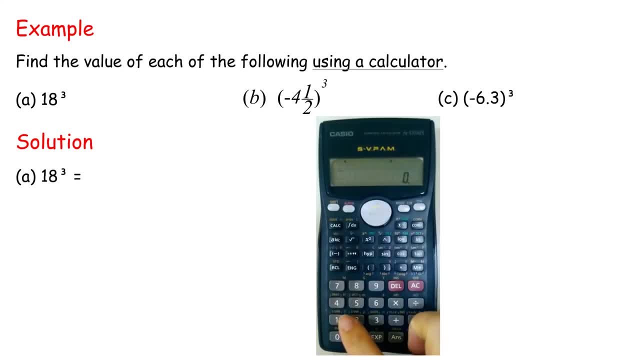 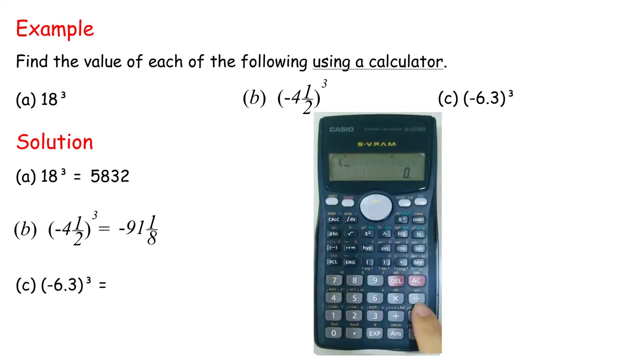 Solution: A: 18 cube equals five thousand eight hundred thirty-two. B: negative four and one over two cubed equals negative ninety-one and one over eight. C negative six point three cubed equals negative two hundred fifty point zero four seven. 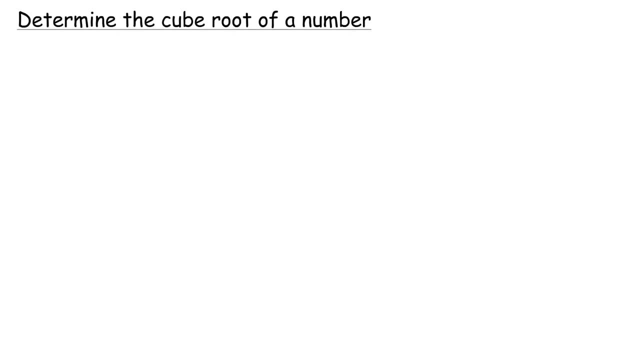 Determine the cube root of a number. Example: Find the value of each of the following without using a calculator Solution: A cube root of sixty-four equals cube root of sixty-four. A cube root of sixty-four times negative four and one over two cubed. 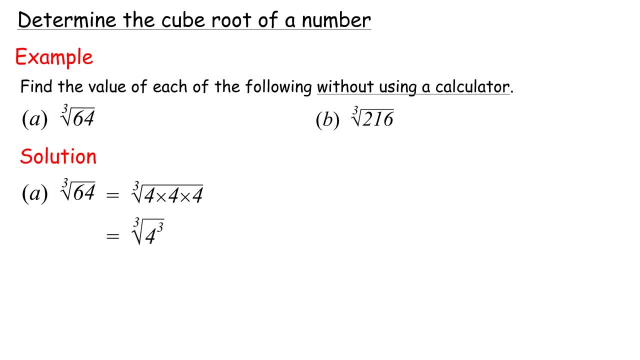 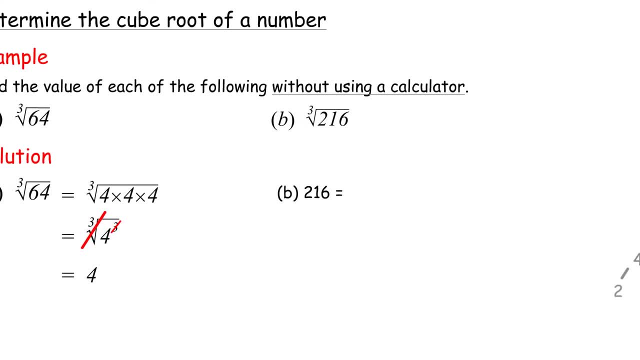 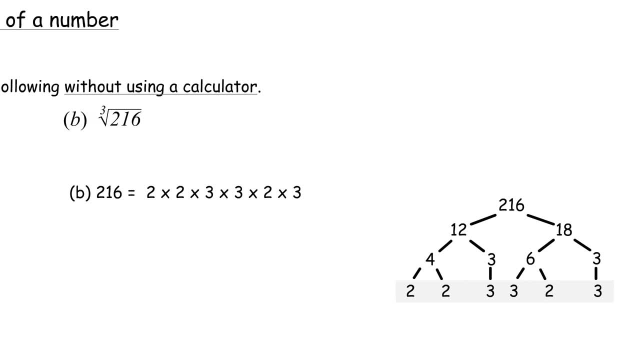 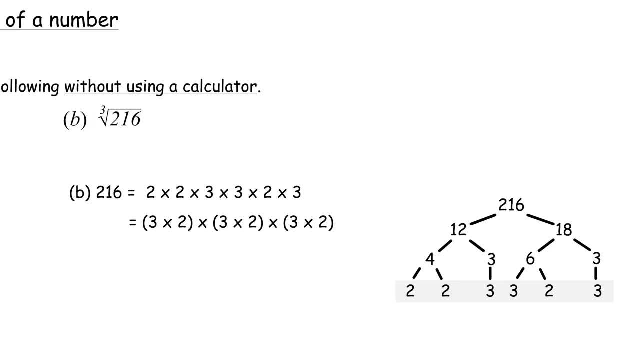 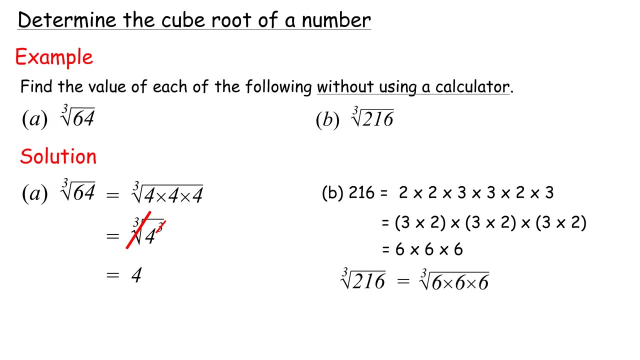 equals negative twenty-one and one over three cubed equals three times two times three times two times three times two equals six times six times six. cube root of 216 equals cube root of six times six times six equals cube root of six cubed equals six. 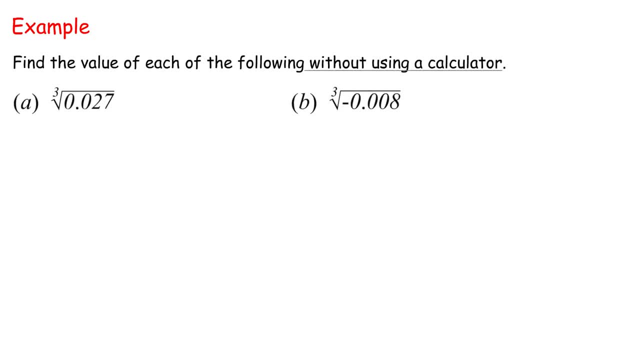 example, find the value of each of the following without using a calculator solution: a. cube root of 0.027 equals cube root of 0.3. cubed equals 0.3. b cube root of negative 0.008 equals cube root of negative 0.2 cubed equals negative 0.2. 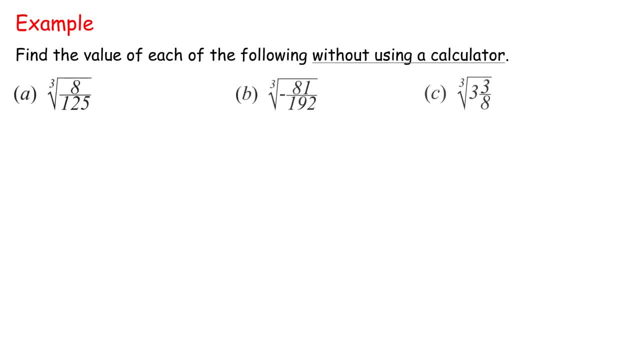 example, find the value of each of the following without using a calculator solution: a. cube root of eight over 125 equals cube root of two fifths times two. fifths times two fifths equals cube root of two fifths cubed equals two fifths. b. cube root of negative: 81 over 192. 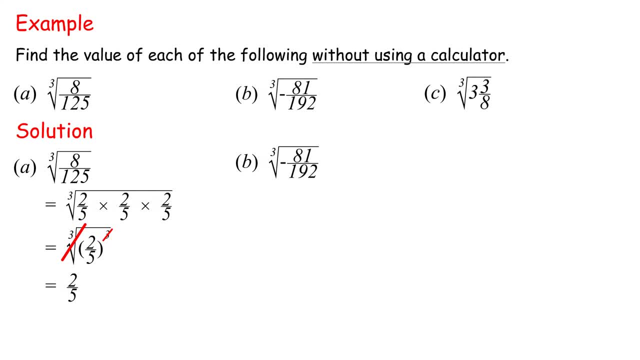 simplify the fraction first: equals cube root of negative 27 over 64. also find the value of each of the following without using a calculator: 4, equals cube root of negative 3 quarters times negative 3 quarters. times negative 3 quarters equals cube root of negative 3 quarters cubed equals negative 3 quarters. 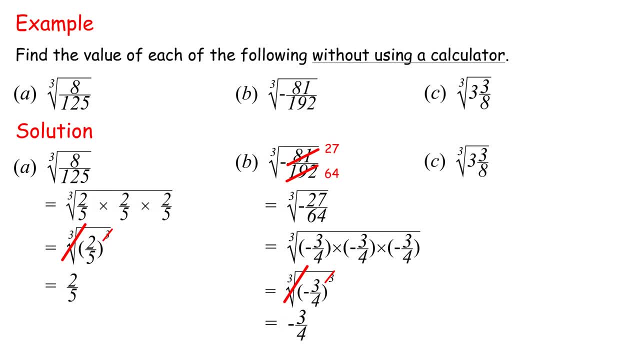 C. cube root of 3 and 3 eighths. convert to improper fraction: first: equals cube root of 27 eighths. equals cube root of 3 over 2 times 3 over 2 times 3 over 2, equals cube. 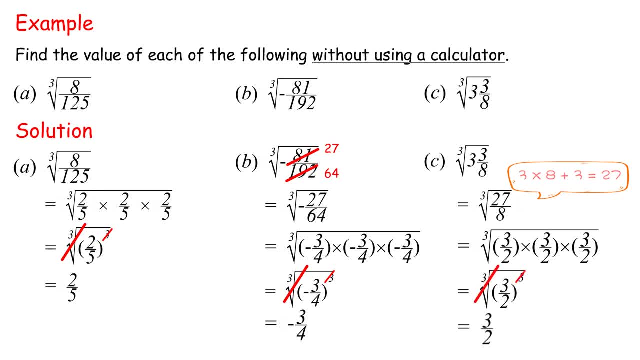 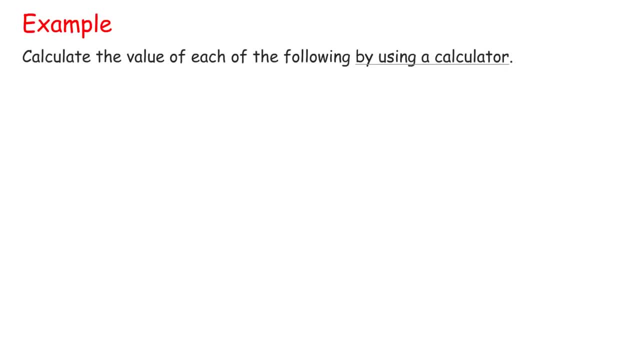 root of 3 over 2 cubed equals 3 over 2, equals 1 and 1 over 2.. Example: calculate the value of each of the following by using a calculator. Give your answer correct to two decimal places.